You look at an artwork and ask yourself: why did this artist use this color? Does it mean something? Could she have used another color? Join us as we uncover three simple steps for analyzing color. Hopefully it'll give you a deeper understanding and appreciation for art. 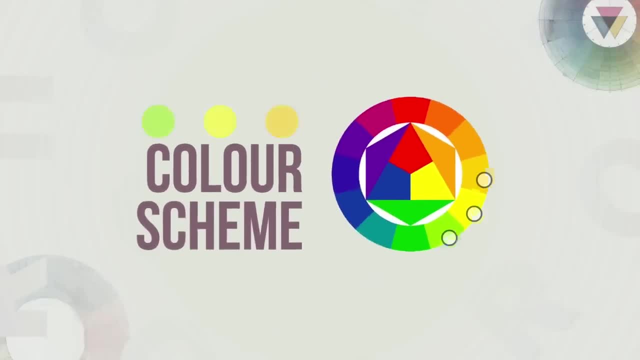 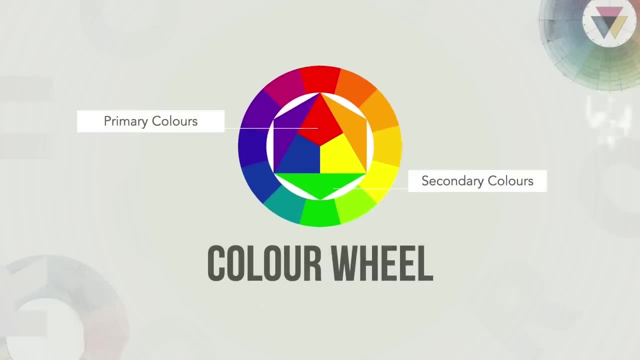 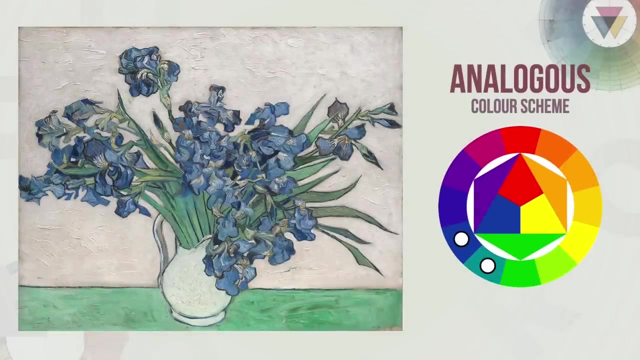 Step 1. Color Schemes. An artwork's color scheme is the carefully selected set of colors from the color wheel. In our demonstration we'll stick to the primary and secondary colors. There are five basic color schemes to consider. First we have the analogous color scheme. 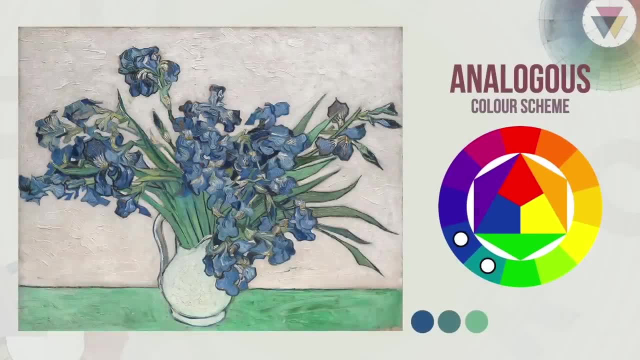 where colors are chosen from the same side of the color wheel. This choice creates cohesion and harmony in the piece. Typically, one color takes the lead, while the other support and enhance the overall composition. Now in this artwork, we see another analogous color scheme. 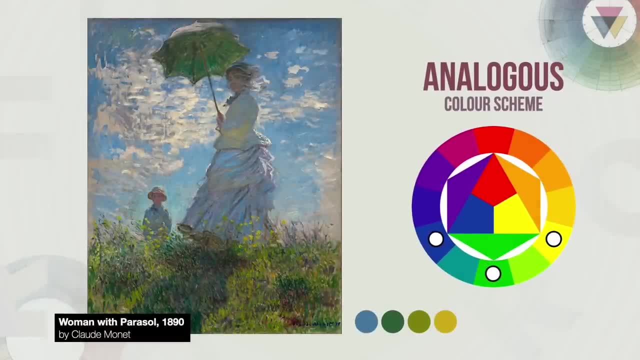 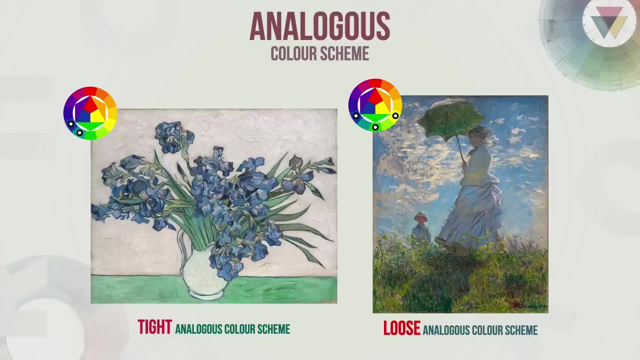 but with colors that are slightly farther apart. We'll use the color scheme to determine the color scheme. This is referred to as a loose analogous color scheme, while the previous one is considered a tight analogous color scheme. Both schemes unify various elements and offer a visually pleasing 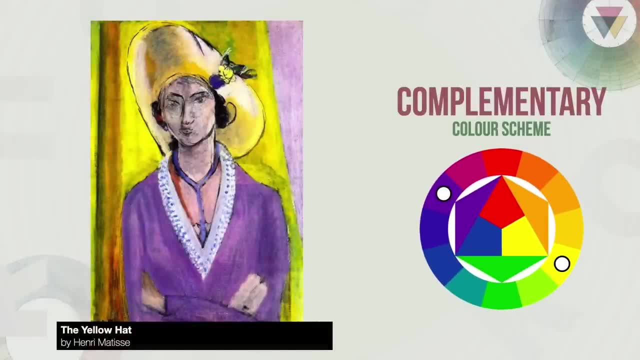 experience. Moving on to the complementary color scheme, where colors are chosen from opposite ends of the color wheel, This pairing creates a striking visual contrast, emphasizing one color over the other. One color usually dominates, while the other plays a supporting role, often in a desaturated or shaded form. 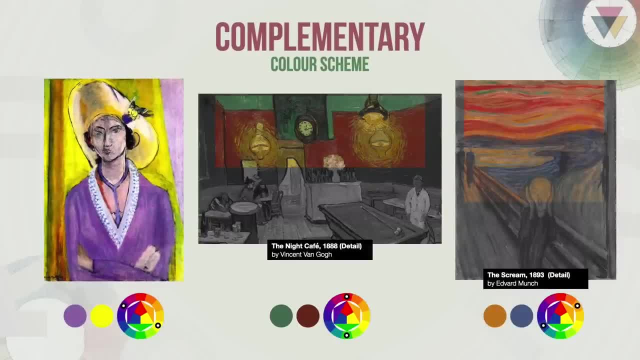 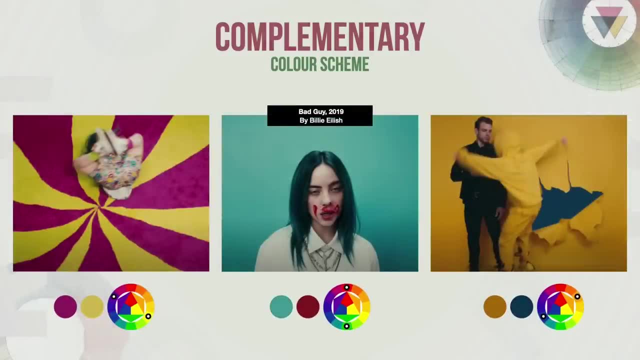 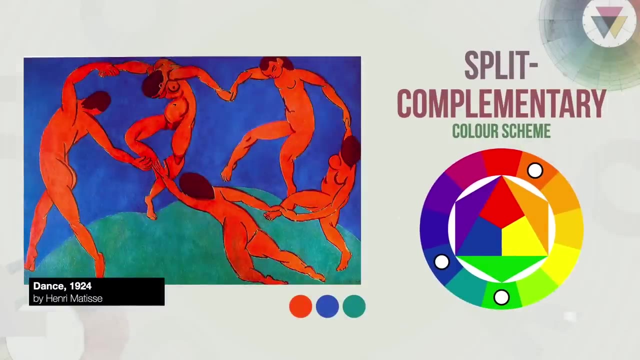 Common complementary pairs include yellow and purple, red and green and blue and orange. You'll notice that many music videos use this color scheme because it is the most eye-catching or visually arresting. An extended version of the complementary scheme is the split complementary color scheme. Here one color is paired with two adjacent colors on the wheel. 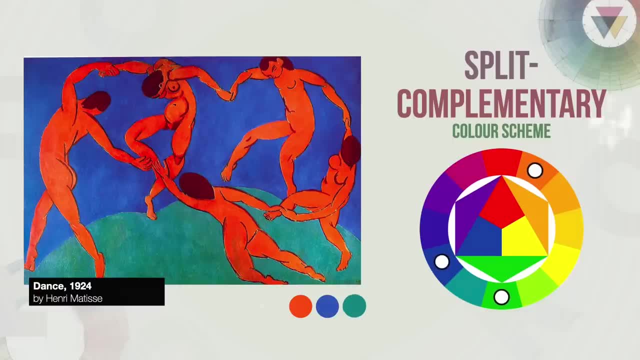 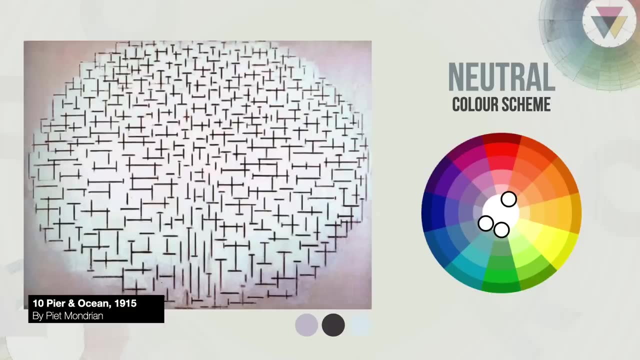 still creating contrast, but with less tension. Our next stop is the neutral color scheme, which uses muted, desaturated colors. These colors evoke a mellow and soft ambience, offering visual rest. However, extreme values like black and white can introduce tension. 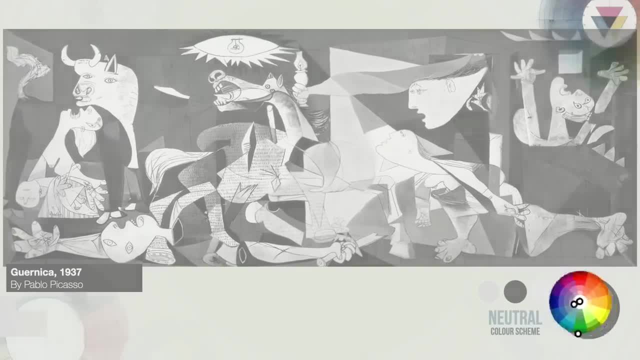 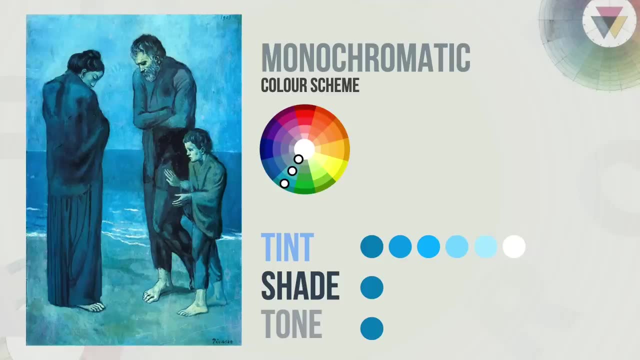 Finally, we have the monochromatic color scheme, which employs a single color in various tints, shades and tones. Tints are lighter versions of color, shades are darker and tones are desaturated. Artists use this scheme to enhance the mood of a scene, expressing emotions such 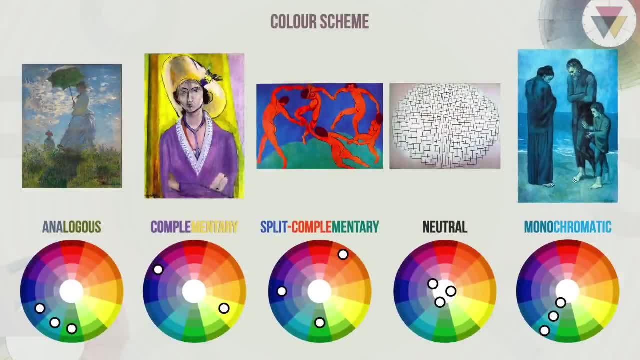 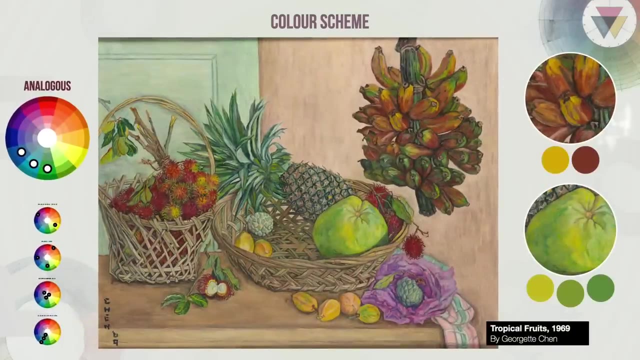 as sadness or joy. These are the five major color schemes to look out for in artworks. They can be present throughout the entire composition or in specific parts of the artwork, For example in this work by Georgette Chen. analogous color schemes can be found in the pomelo and the ripped bananas on the 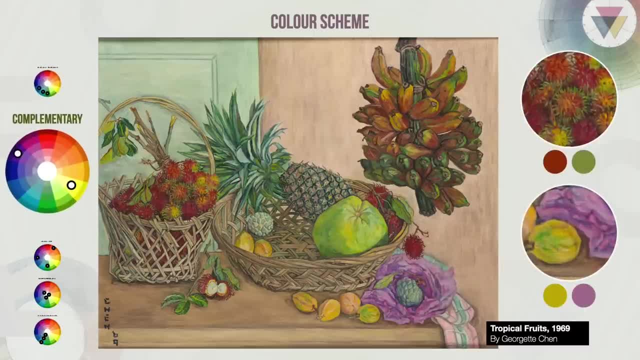 top left corner, while complementary color schemes are found scattered throughout the artwork, such as the red and green rambutans against the green door or yellow fruits in the right foreground juxtaposed with the purple wrapper. She also employed a neutral background to allow. 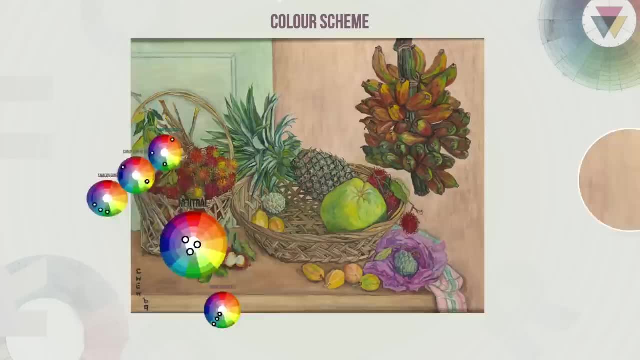 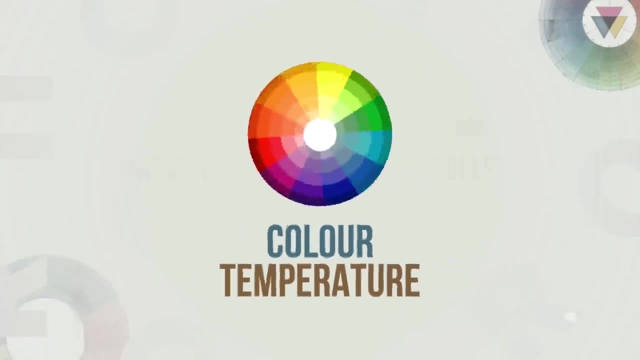 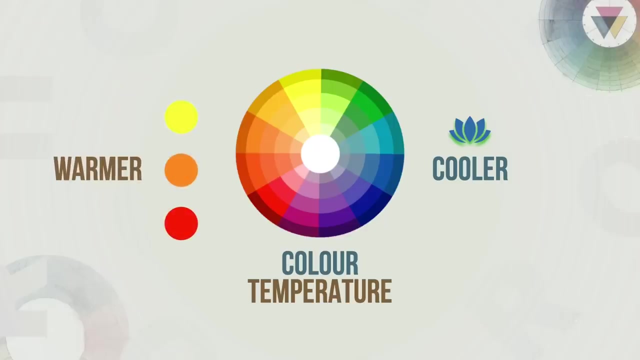 the more saturated fruits to stand out. Can you find other color schemes In this artwork? step to color temperature. color temperature divides the color wheel into warmer and cooler categories. Warmer colors are associated with fire, So yellow, orange and red. They tend to advance toward the viewer, meaning they appear closer to 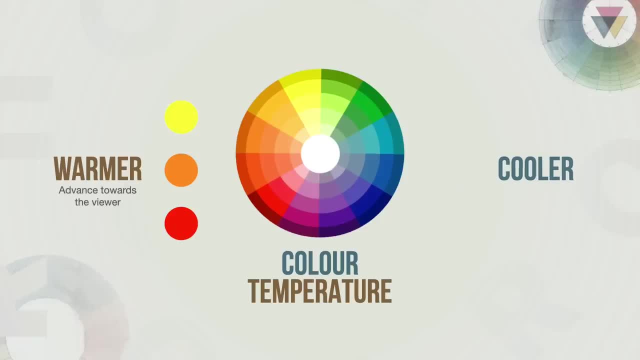 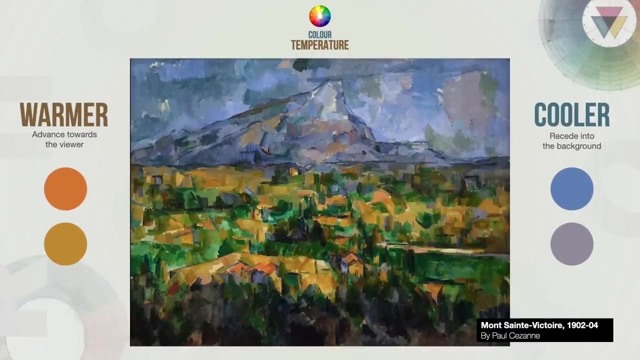 you, While cooler colors associated with water and greenery- So green, blue and purple- recede into the background, they appear to be further away from you. in this artwork by post Impressionist artists frågor Zan dominate the foreground, creating a sense of depth against the cooler mountainous background. 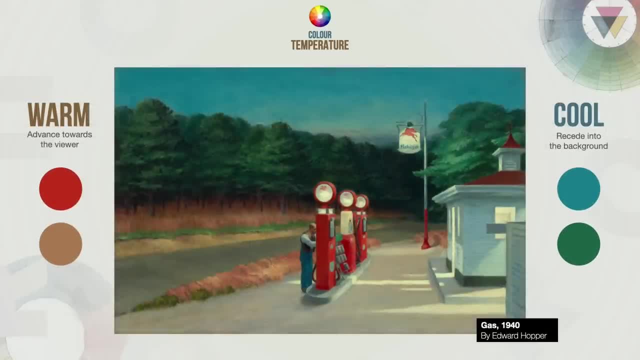 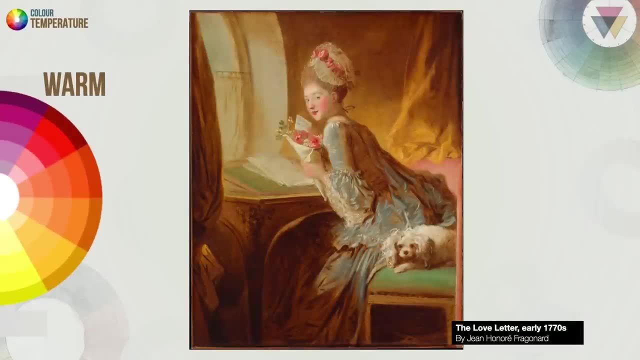 American artist Edward Hopper also employed this technique. Singaporean artist Liu Kang did the same. Color temperature can also evoke different emotions. Warmer color palettes can evoke strong emotions of joy, like this artwork by French painter Jean Fragonard, while cooler color 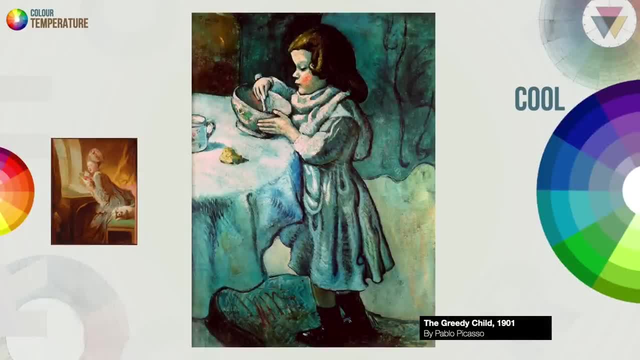 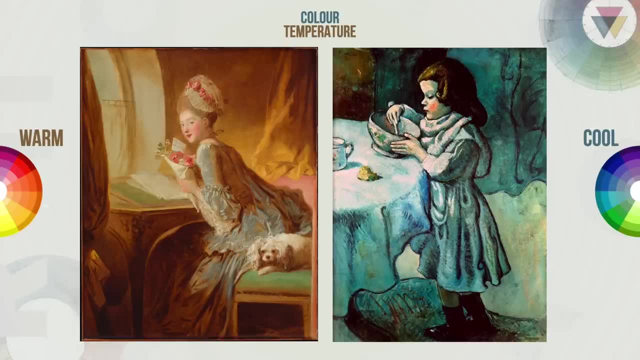 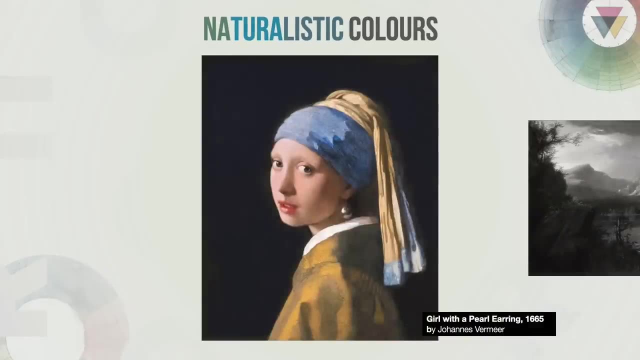 palettes suggest calmness, tranquility or melancholy, like this work by Spanish painter Picasso. Do you like to use warm or cool colors? Share your preference in the comments below. Step 3. Naturalistic vs Unnatural Colors. We can analyze whether the colors in the artwork 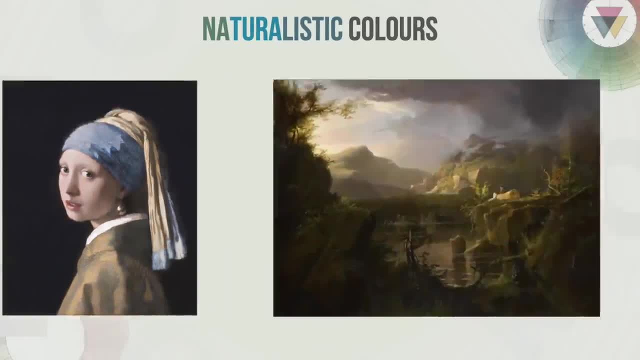 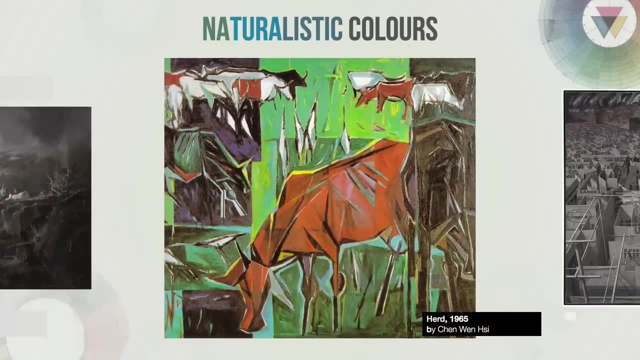 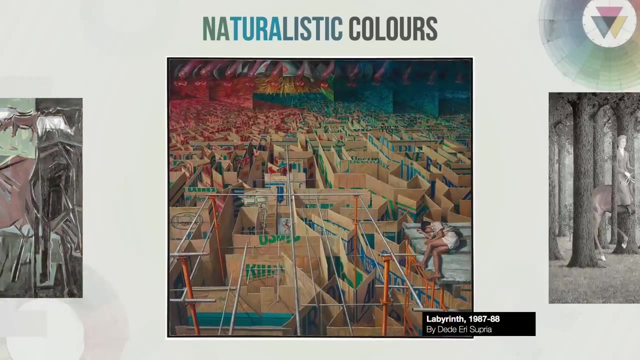 are naturalistic or unnatural. Naturalistic colors mimic reality with green leaves, blue skies and appropriate skin tones. These descriptive colors make the artwork accessible and relatable, even though the subject matter may be distorted. Naturalistic colors also help the viewer to focus on the story being communicated and believe that what they're. 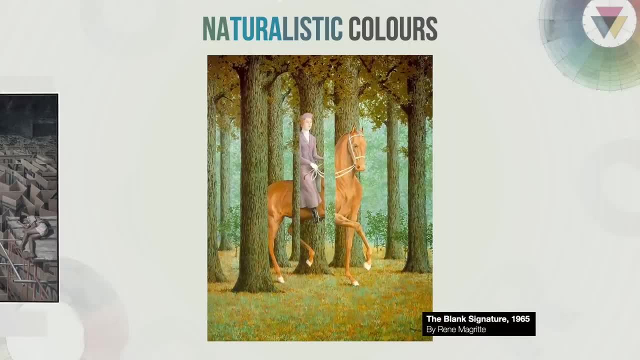 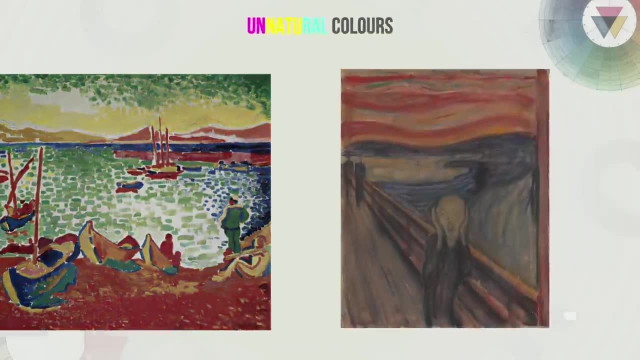 seeing is in fact real, even though they may not be so. On the other hand, unnatural or abstract colors convey the artist's subjective understanding of the world, using colors symbolically. For example, Norwegian painter Edvard Munch used harsh, reds and oranges to express anger.